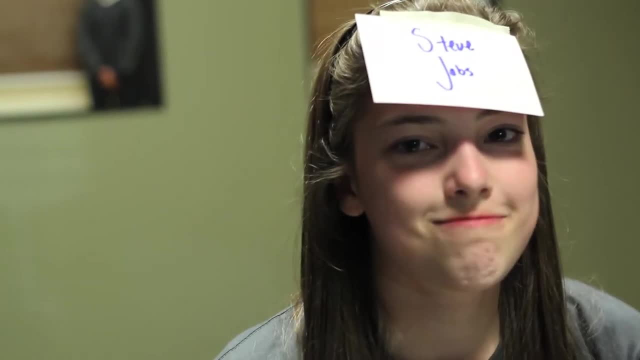 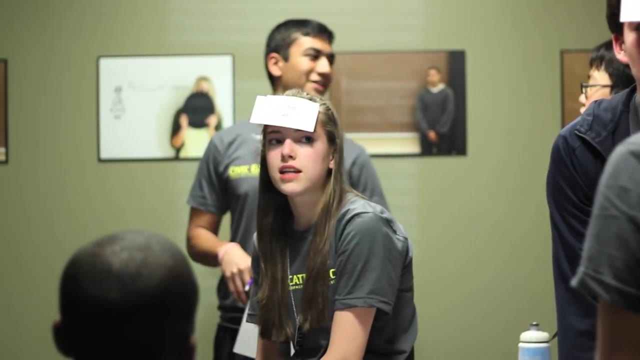 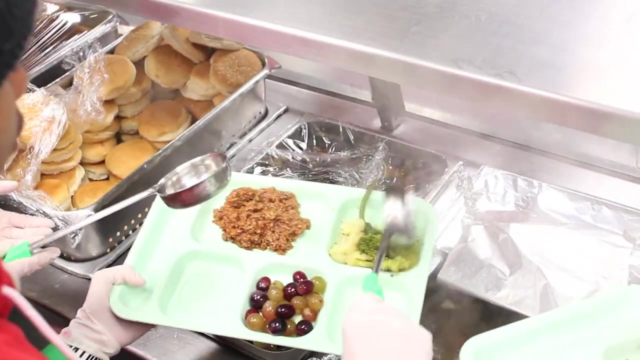 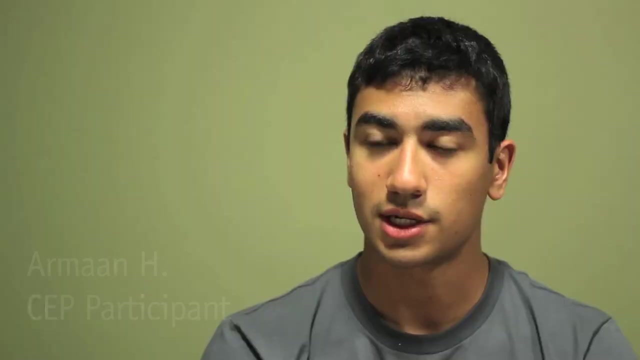 a marriage between academic instruction and learning And experiential learning. We talk to doctors and we talk to people at clinics, like health clinics. There's a lot of different ways that we learn things. We got to see something that we live around but we never even pay attention to. 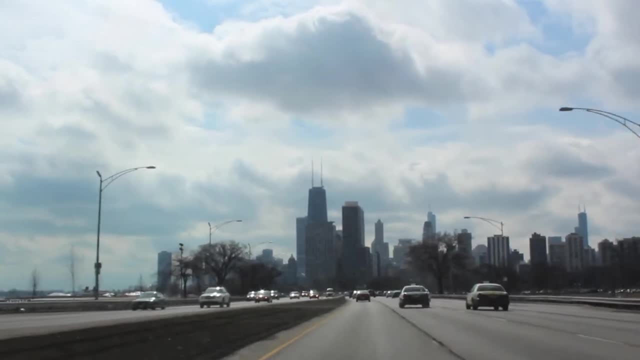 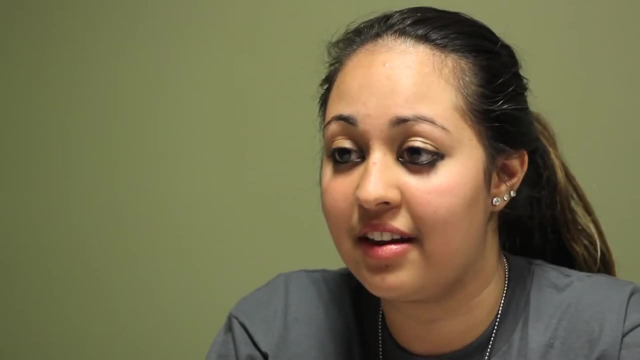 I live in Illinois And I was really, really surprised to see that so many of the things that happened outside of the United States happened just 45 minutes away from where I live. I never really felt challenged and didn't really have that many peers that themselves were interested in school. 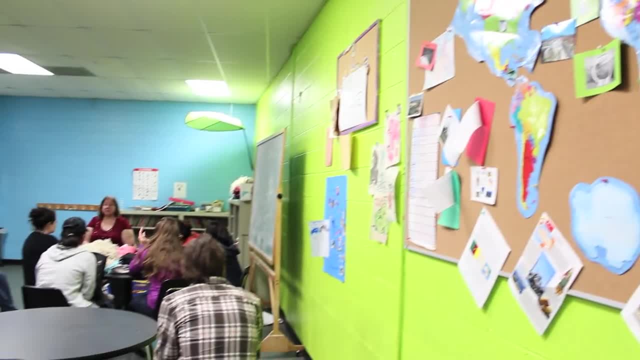 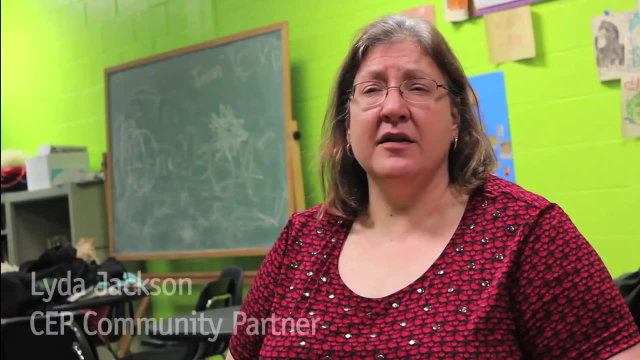 So, coming to CEP, there's a lot of kids who were actually interested in what they were doing, really passionate, and for me that was amazing. I had never experienced that before- ever, I think- just to bring a group of students that are so diverse as the Civic Education Project. 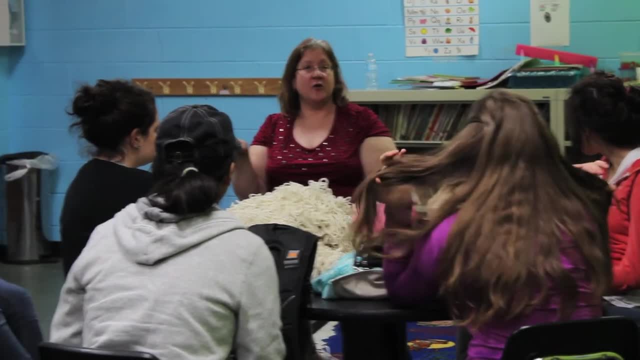 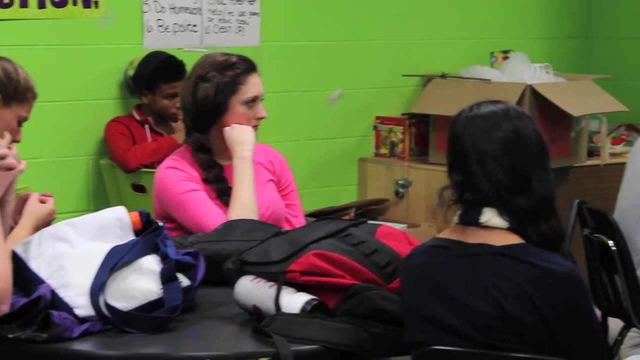 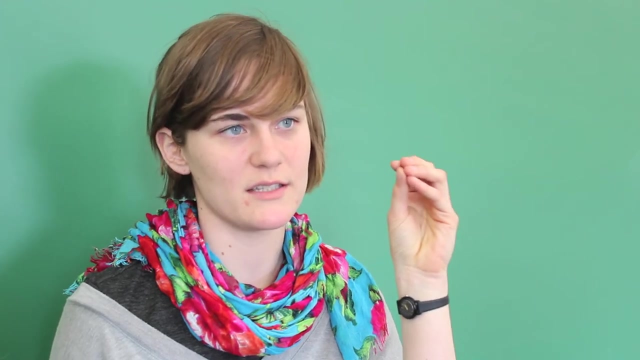 brings together and helps them to cooperate for the duration of the program is very, very valuable and something that these students will take with them wherever they go for the rest of their lives. I think having that critical lens, and getting it when you're 15,, 16,, 17, can make a world of difference for students. 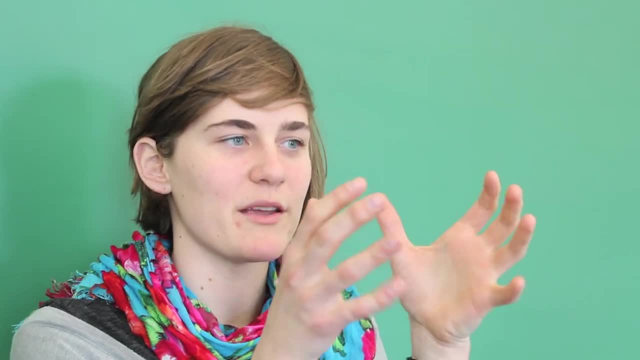 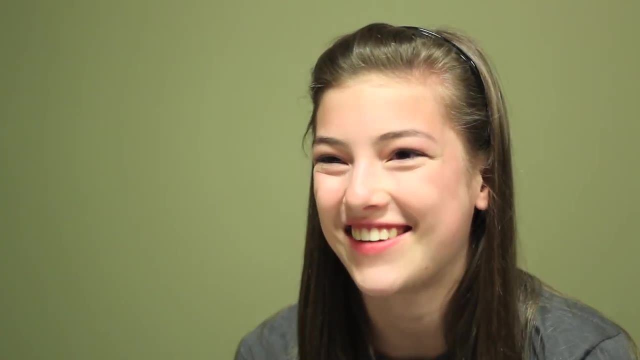 And so I just think it takes wherever you are and it makes you a little bigger, It opens you up a little bit wider. This is something you'll never, ever get to do anywhere else. Yeah, I would definitely recommend it. This program is eye-opening. It's a great way to spend my spring break. 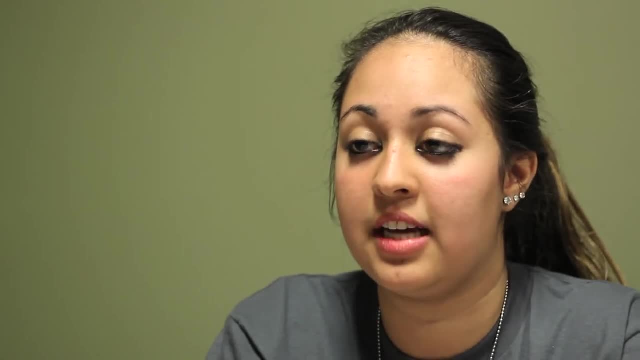 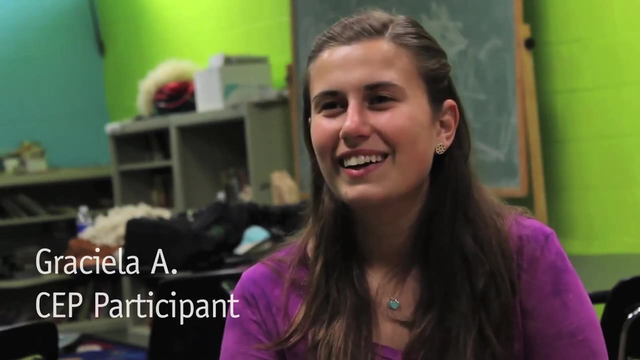 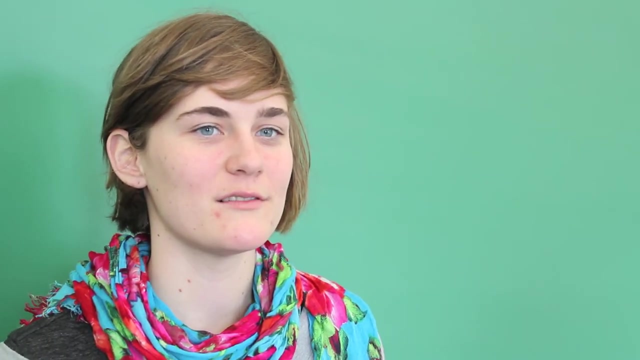 There's already many volunteer sites that I know I can tell my school about and maybe even start a club. I would definitely recommend it to everybody I know because I've had an amazing time and it's just been two days. I think if you're looking for an engaging and meaningful experience, CEP's it. 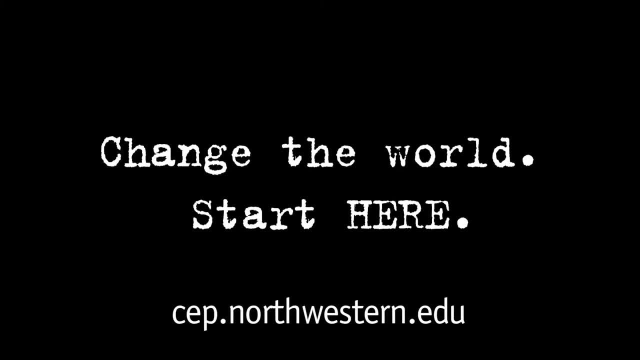